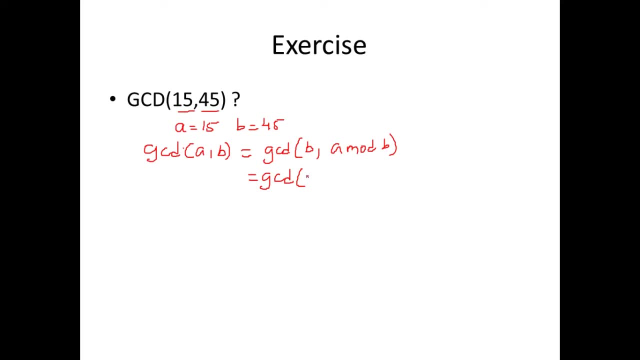 is nothing but gcd of what is b here? 45, a is 15 mod b, that is 45. So what we arrive at here is gcd of 45. What is 15 mod 45? It is just So again we have to use this formula here. So this is like GCD of A comma B. So our 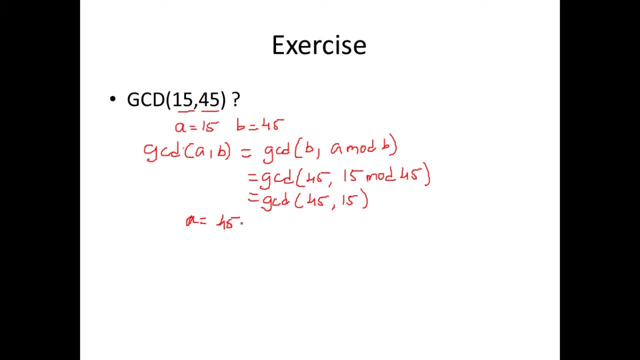 A now is 45, and what is our B? B is 15.. So GCD of A comma B is equal to GCD of B comma A mod B. So we can very well write this as say GCD of 45 comma 15.. So this is of the 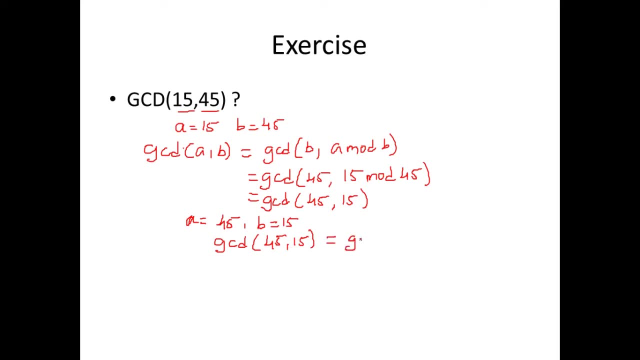 form: GCD of A comma B. This can be written as GCD of what is B. here B is 15 comma, A is 45 mod what is B: 15. This is nothing but GCD of A comma B. So we can very well write. 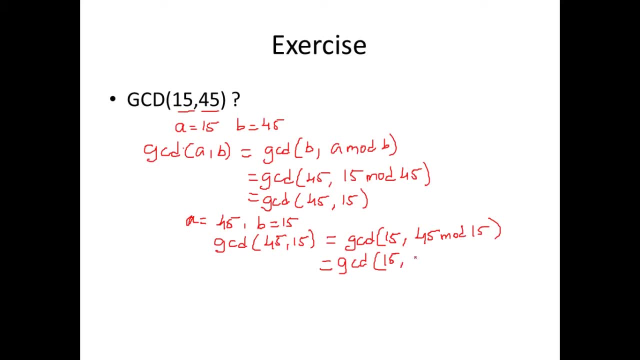 this as 15 comma. what is 45 mod 15?? The remainder is 0. So what is GCD of A comma 0? That is equal to A, So we say 15.. So 15 is the greatest common divisor for 15 and 45. So how did? 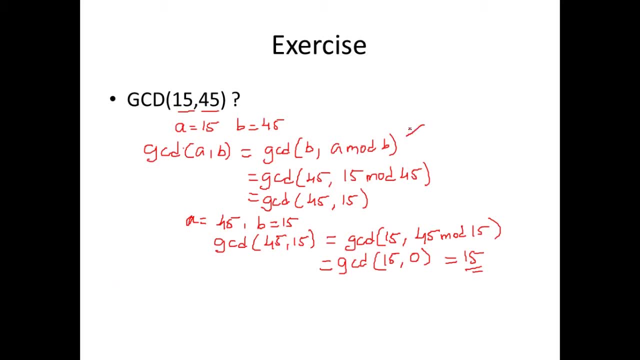 we achieve this? We were achieving this by using this concept repeatedly, So we first found GCD of 15 comma 45. This was equivalent to GCD of 45 comma 15.. GCD of 45 comma 15 and finally, that was leading. 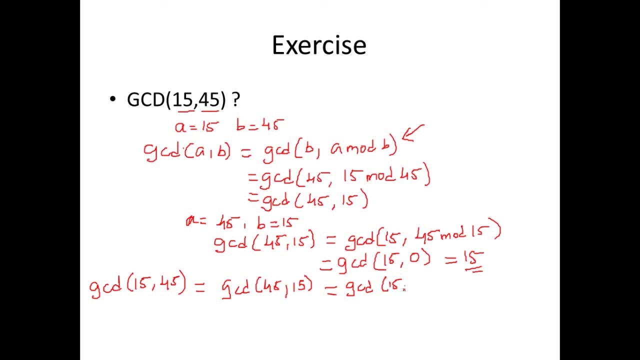 us to this particular value, GCD of 15 comma 0, and finally we arrived at 15.. So we say GCD of 15 comma 45 is nothing but 15.. So this is how you use the Euclidean algorithm to find the greatest common divisor. Let us 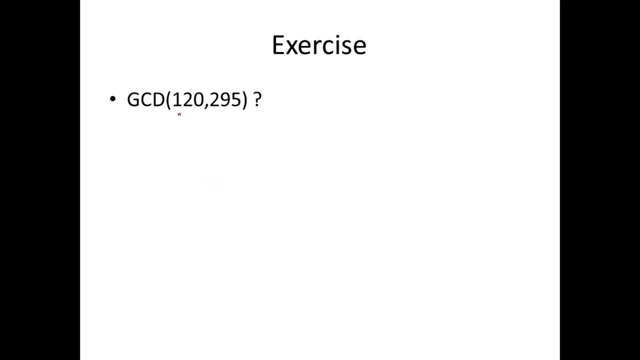 take another example. I want you to compute the GCD for these two values. We have already seen the algorithm. We have taken an example. we understood it. Please go ahead and compute the GCD for this. So here A is 120 and B is 15 comma 0.. So this is the GCD of GCD of 45 comma 15.. So 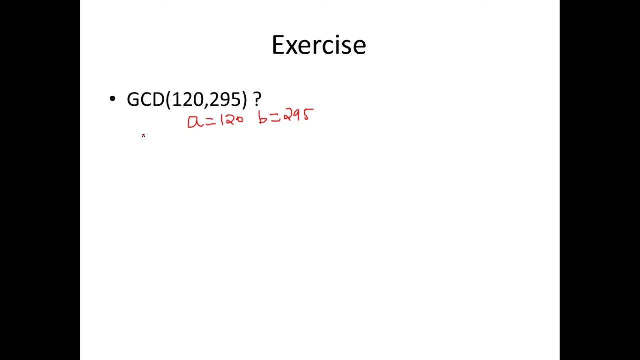 B is 295.. So what is GCD of A comma? B is nothing but GCD of B. What is B 295 comma? A mod B? that is 120 mod 295.. So this leads us to GCD of 295 comma. what is 120 mod 295?? 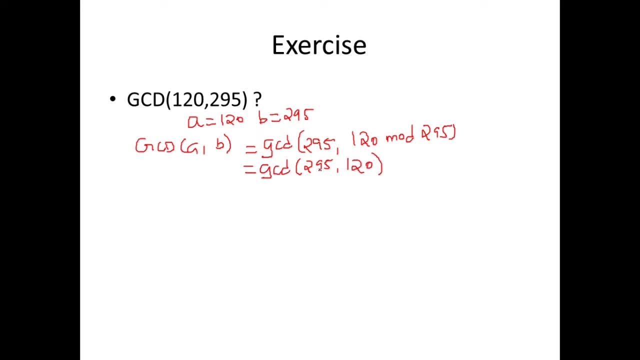 It is 120.. So now we have this in the form GCD of A comma B. What is A here, This is 295, and what is B here, That is 120.. So now we can write this GCD of 295, comma 120 can. 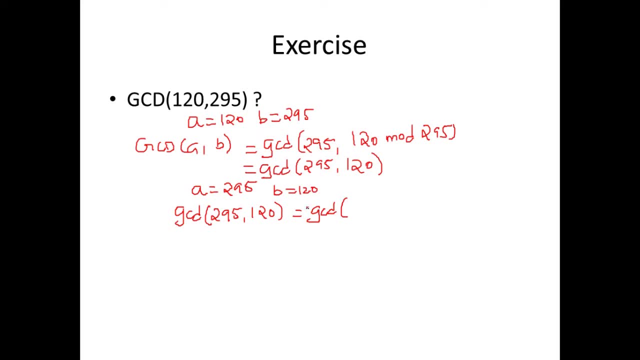 be written as GCD of B. What is B? B is 120 comma. B A mod B, that is 295 mod 120.. So what is the result here? This is GCD of 120.. What is the remainder when you divide 295 by 120? 55.. So it is 55.. So now our A is new A. 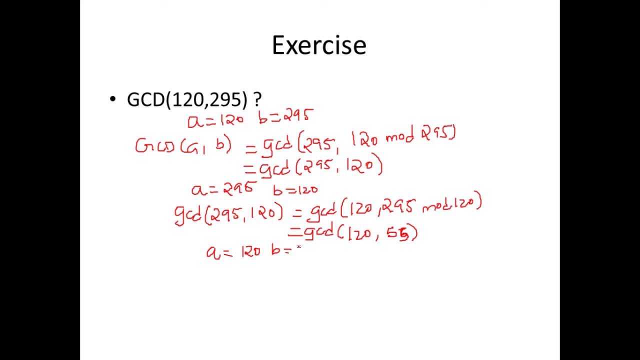 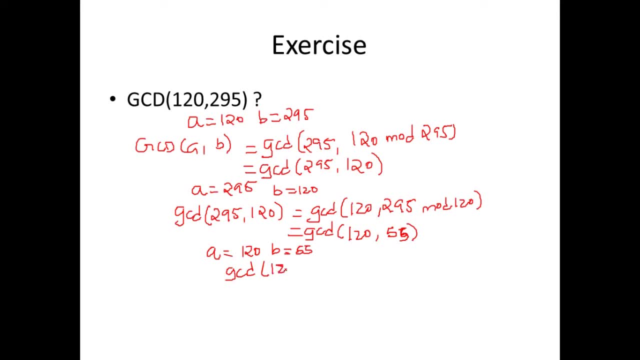 GCD of 120.. So now we can write this GCD of a, that is 120 comma, B 55, as we can just write it as GCD of B, that is 55 comma, GCD of a mod B, that is 120 comma 120. 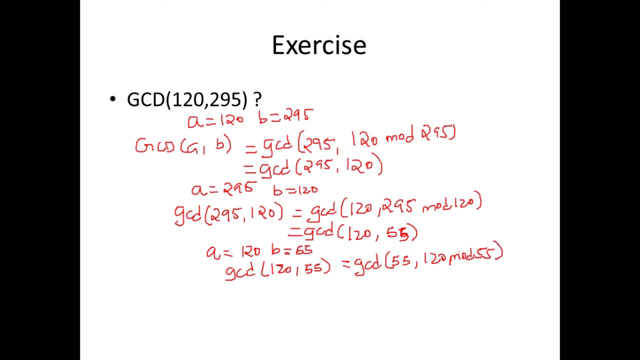 more 55.. So what is the result we get here? This is GCD of 55.. What is GCD of A mod B? This is GCD of 55.. What is GCD of B, 50 more B plus. Now, what do we get? This GCD. 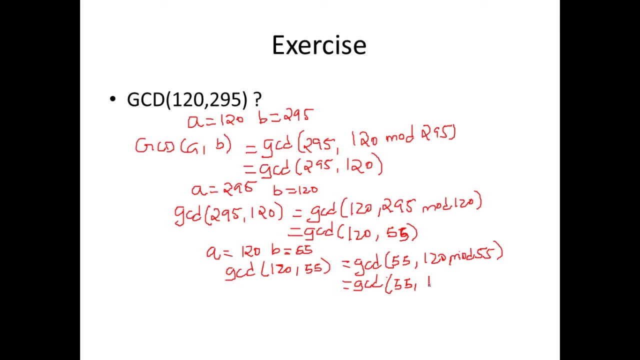 of B plus is less or minus, or plus 1 or minus of B plus minus 0.li. Why is A less or 120 divided by 55? the remainder is 10.. so again, let's continue the process. now. a is 55. what is b? 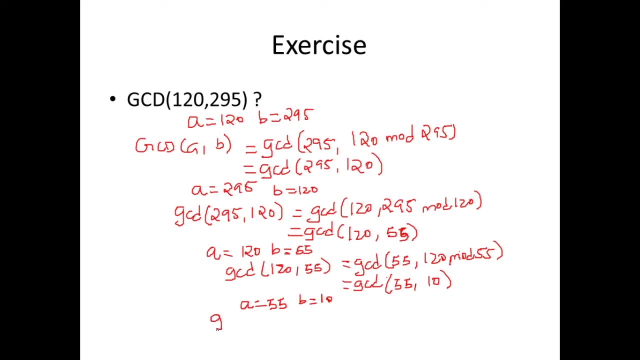 b is 10.. now we can write gcd of 55 comma. 10 a comma b is nothing but gcd of 10 comma. so that is 55 mod 10.. so what is this? this is nothing but gcd of 10 comma. what is 55 mod 10 when you divide? 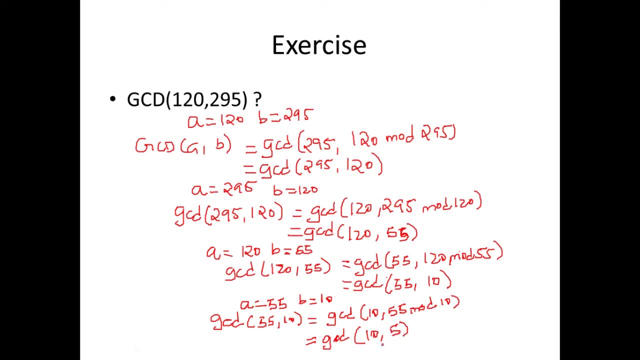 10 by 55, the remainder is 5.. we have not yet achieved 0 here. we have to continue this process until b goes to 0, so we will continue this. i have been continuing this year. so what we have achieved is gcd of 10 comma 5.. 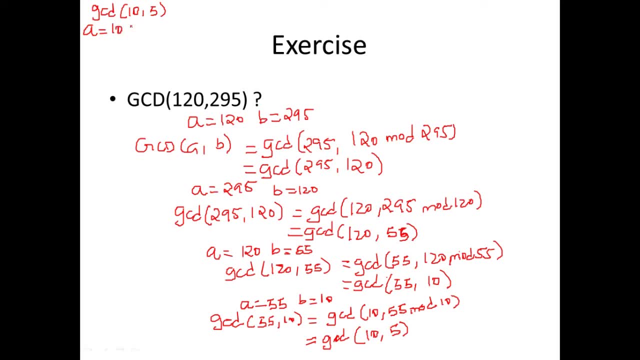 so now our a is 10 and b is 5.. so we can write: gcd of a comma b is nothing but what is this? this is gcd of b, 5 comma, a mod a mod 5. that is a mod b. so this is nothing but gcd of 5 comma. what is 10 mod 5? 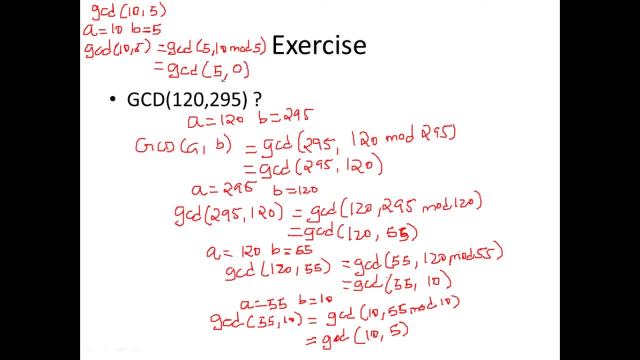 remainder is 0.. so now we know gcd of a comma 0 is equal to a, so we say 5 and then we terminate the process. since we have reached 0 here, we will terminate the process, and what is the output? 5.. the best common divisor for 120 and 295 is 5.. i hope you are able to follow this. 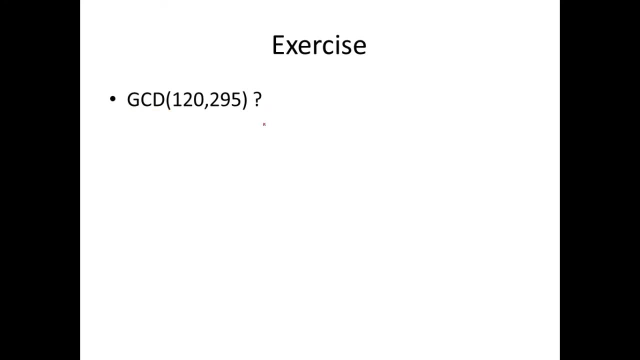 so we will see another way of writing the same concept. according to the division algorithm. we know this. when a is divided by n, a can be very well written as: a is equal to n into q plus remainder r. So this is the division algorithm. we have learnt this in our previous classes, So we 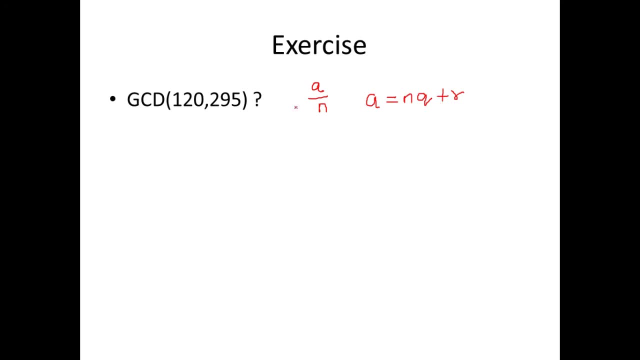 can use this concept and we will be able to find the GCD. So let me tell you how to use that. So we will take the greatest number here and assume it as a, and this number is considered to be n. We will represent this in the form given here. We will divide a by. 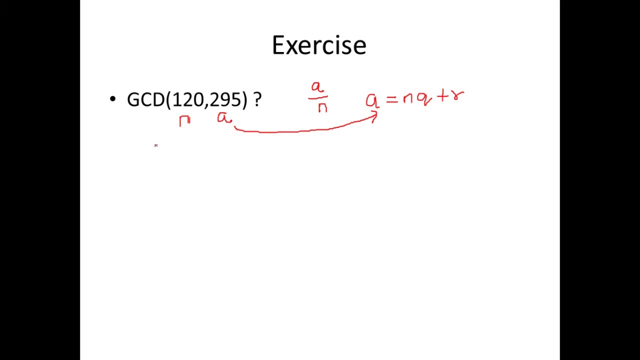 n and we will represent it in the form given here. So 295 is equal to 120 into 2. So that is 240 plus reminder 55. So it is nothing but 295.. We are expressing 295 using this. 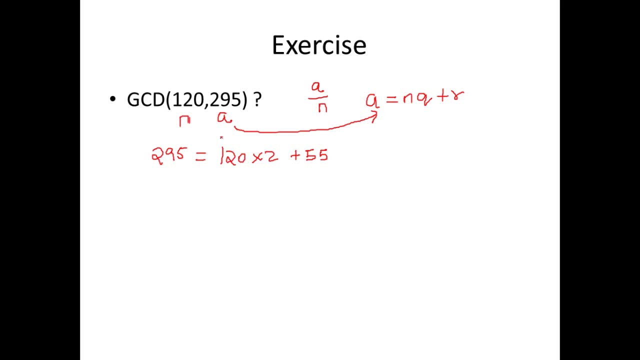 concept a is equal to n cube plus r, So it is nothing but 120 into 2 plus 55. Or else we can even write this as: 295 by 120 can be represented like this: That is nothing but 120 into 2 plus 55.. The next thing is, we are going to take 120 here and we are going 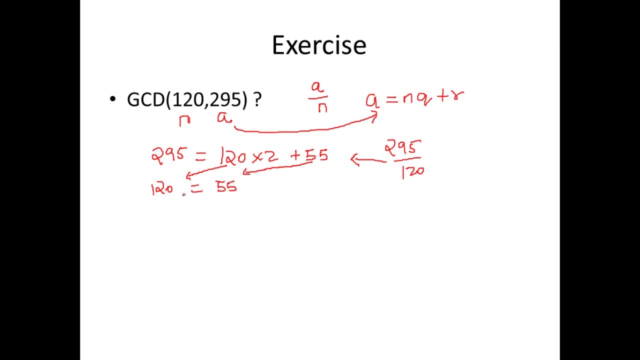 to take the reminder 55, and we are going to represent 120 in the format given here using this. So 55 into 2 is 110, the reminder is 10 and now we will take this 55. here 55 is equal. 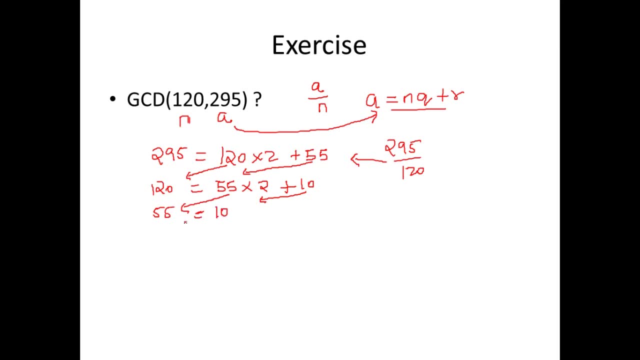 to. we will take the reminder 10 and 10 into 5 is 50. So the reminder here will be 5.. That is the next step. Next step, we will be moving 10 here. So we will be expressing: 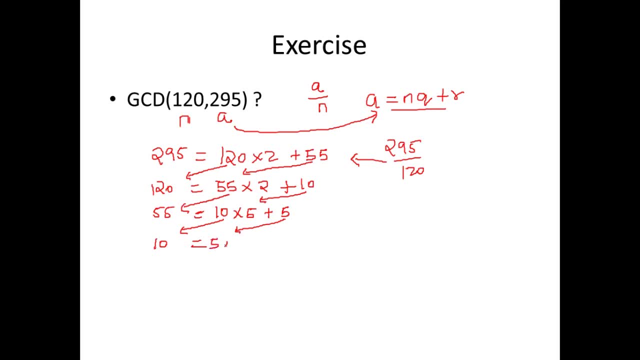 10 using the reminder 5.. So the reminder is nothing but 5 into 2 plus reminder is 0. So once when you reach 0, we stop here. The reminder we have achieved in the previous step, 5, is considered to be.